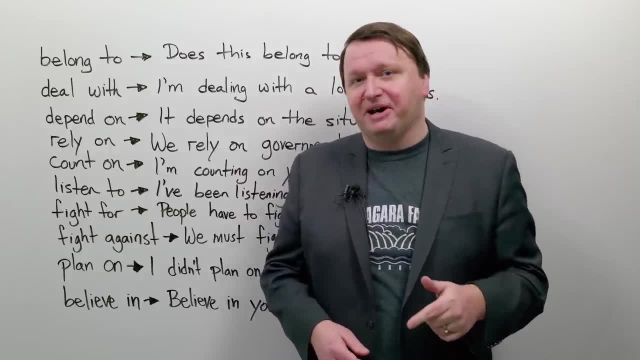 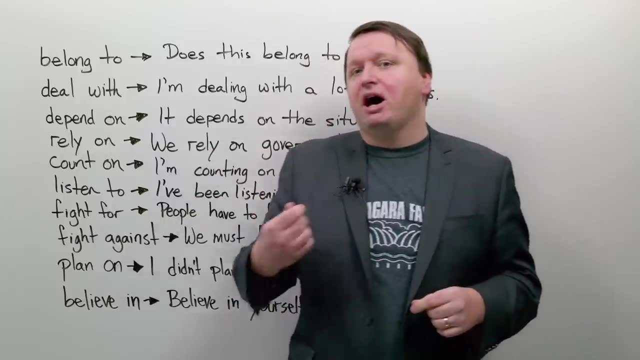 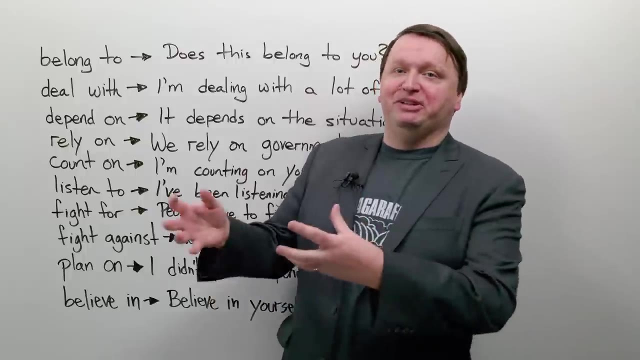 also make sure to check out the quiz on engvidcom. Now let's take a look at some prepositional verbs. We start with belong to, So you can belong to a group or belong to a family or something like that. So belong to a church, belong to a mosque, for example, Does this belong? 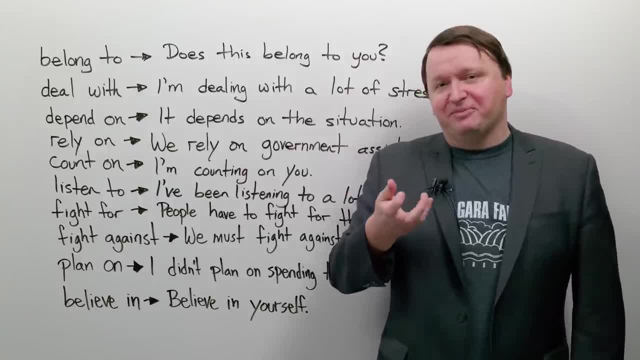 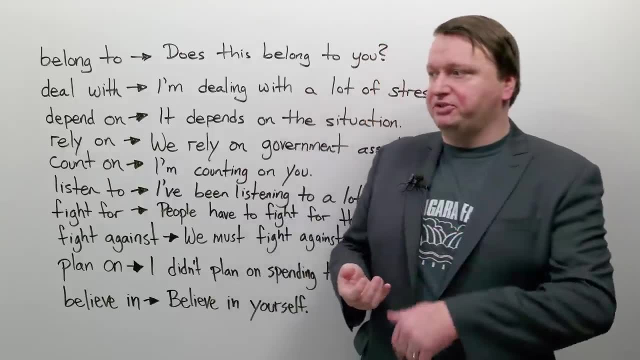 to you. So you are asking if someone is the owner, the possessor of something. So if you found a phone and you think it belongs to Tina, you can say: hey, Tina. You can say: is this yours Or? 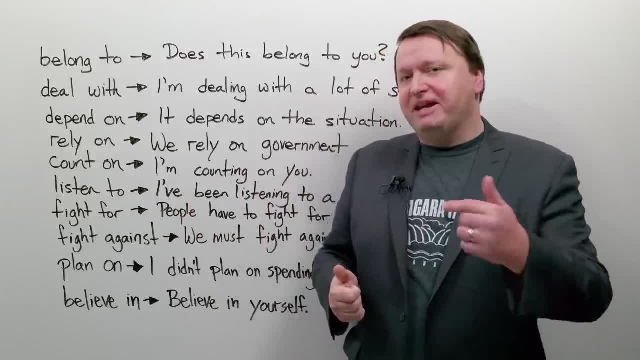 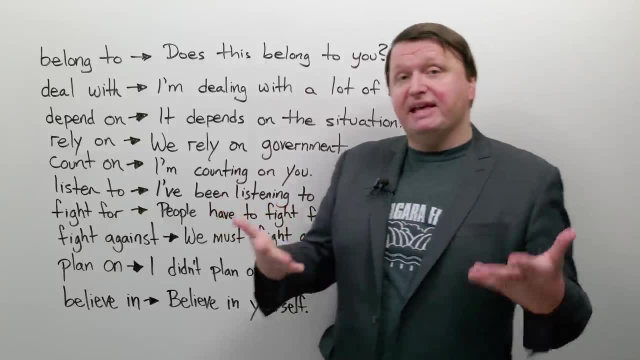 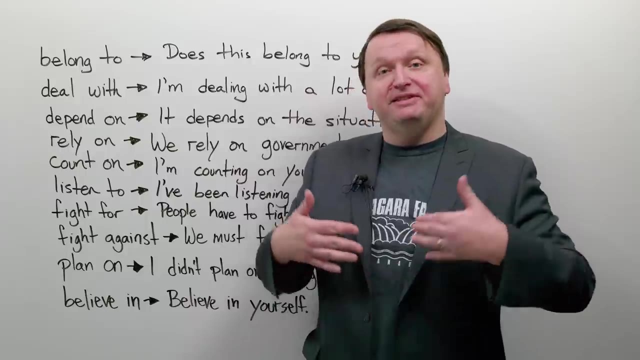 does this belong to you? So repeat after me: Does this belong to you? Good, It's like asking: is this yours So you can deal with people, deal with problems. How you deal with things is how you manage them. 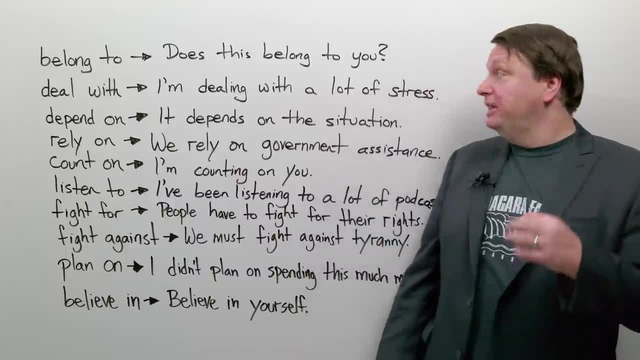 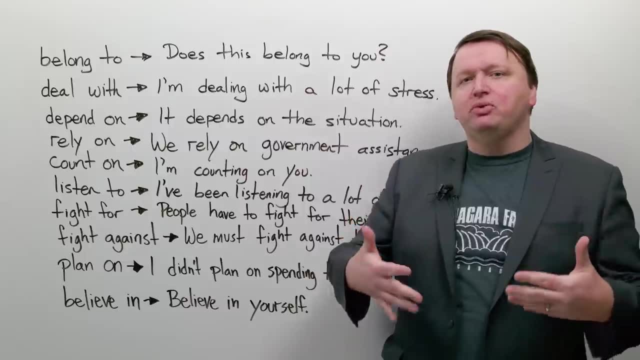 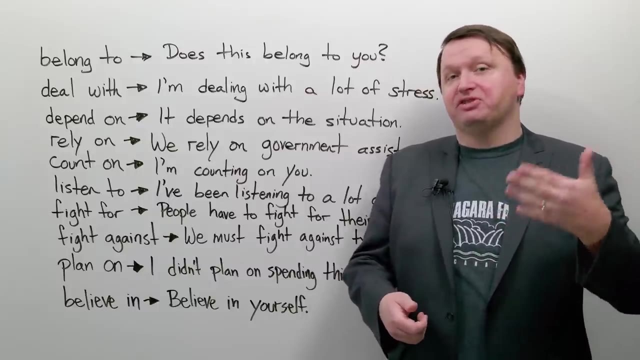 So, for example, I am dealing with a lot of stress. So this means you currently have a lot of stress in your life and you are doing your best to manage it, to handle it. So I hope you are not dealing with a lot of stress these days, But just in case, if you have a lot of stress, 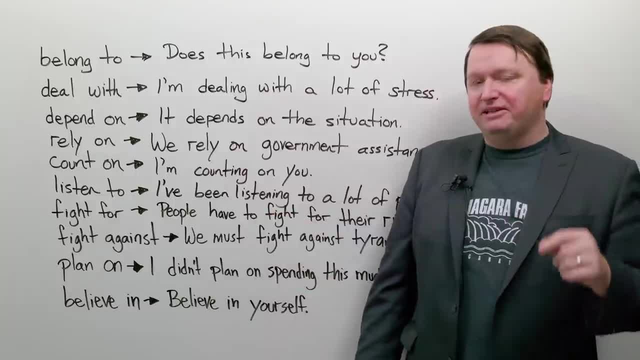 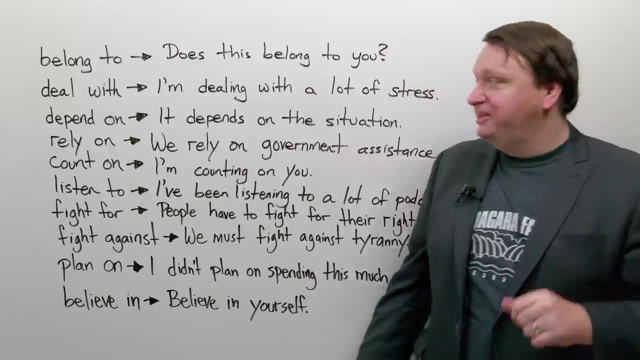 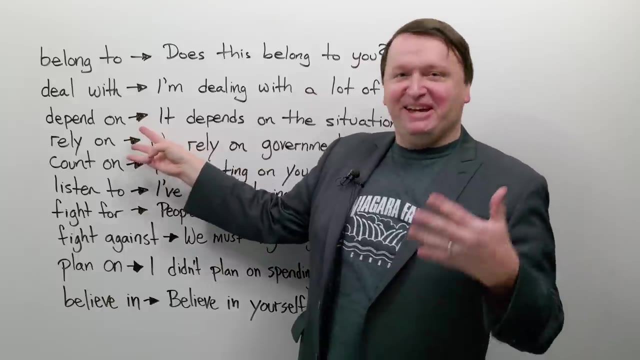 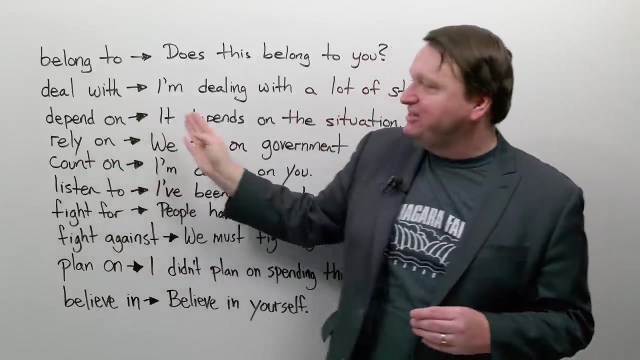 let's repeat this sentence after me. I am dealing with a lot of stress. Good, Next we have this. I am going to call this the trifecta of dependence. A trifecta means there are three. You hear the word try. So the trifecta of dependence with depend on, rely on, count on. 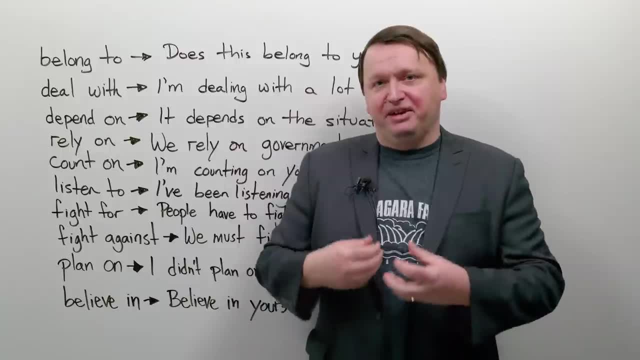 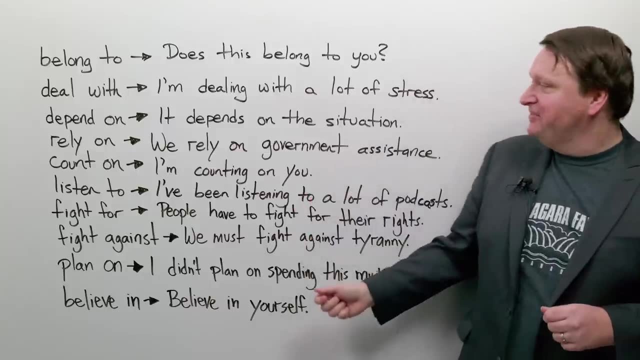 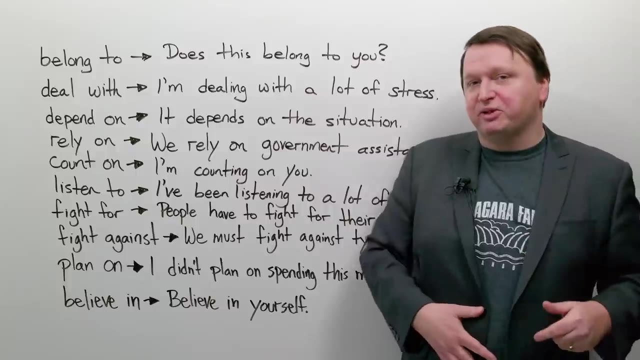 So this means you need someone or something in order to accomplish something, or you need them in order to continue living in some cases. So in this case, a very common mistake is depends of. I've mentioned this in previous videos, so I'm going to mention it here again: It depends on the situation. 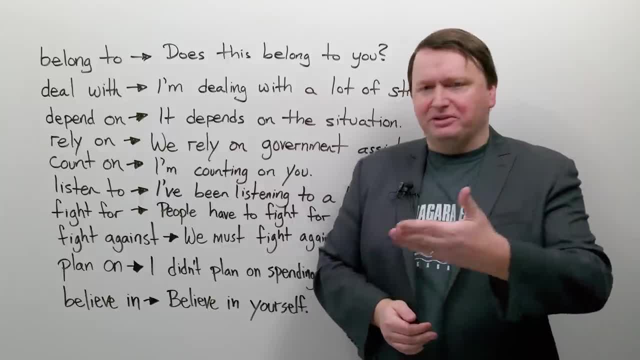 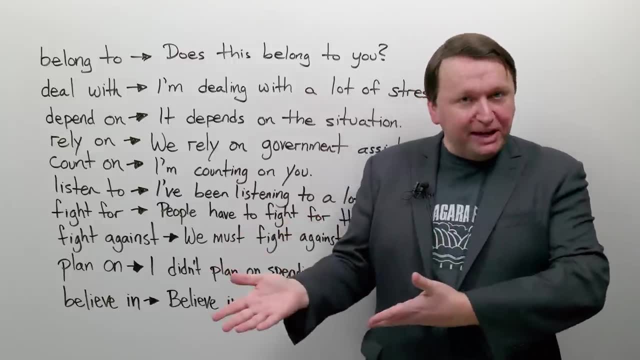 So if I say, oh, would you do this or that, Or do you think this or that, And you can say, well, I don't know, It depends on the situation. So repeat after me this very common sentence: It depends on the situation. 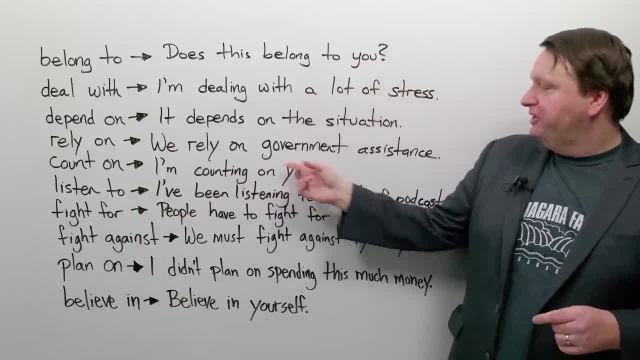 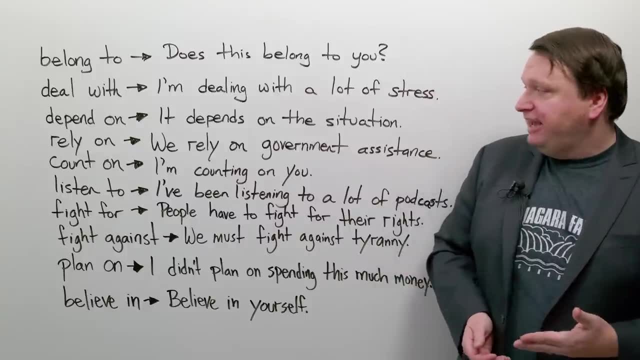 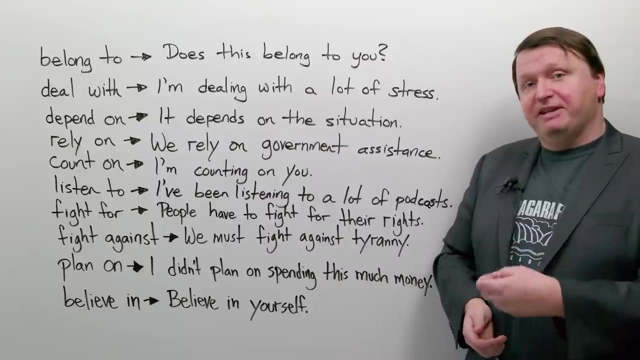 Good, Rely on. So, for example, maybe you are having a rough time, Maybe you have lost your job recently and you are relying on government assistance. So here we have the sentence: we rely, Rely on government assistance. This is similar to: we depend on it. We need it in order to continue. 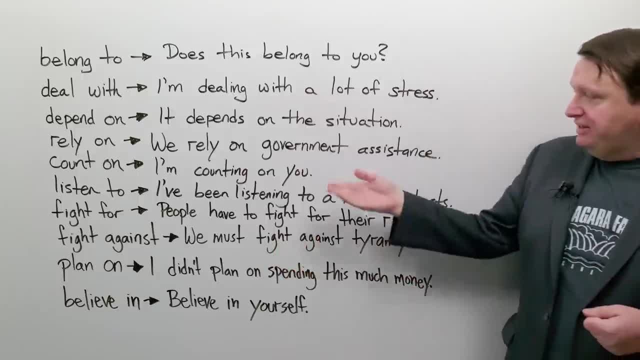 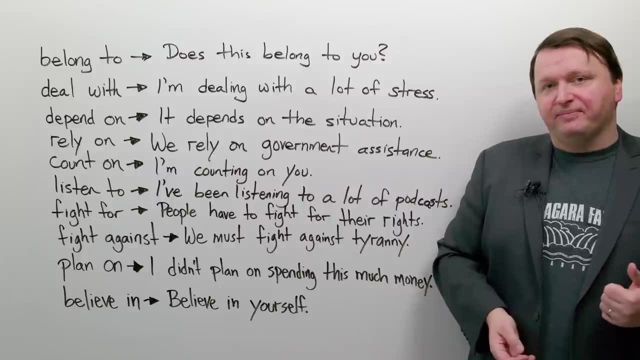 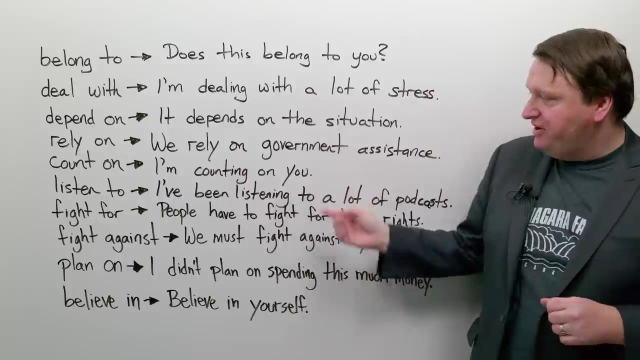 paying for our house to receive money. So you need the government assistance in this case. So repeat after me: We rely on government assistance. Good Count on This one is very common. This sentence in particular. just repeat it after me. 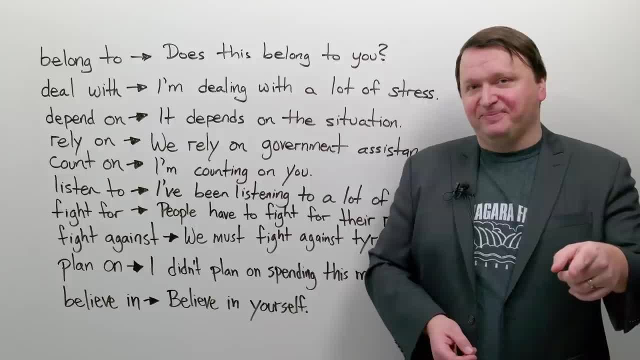 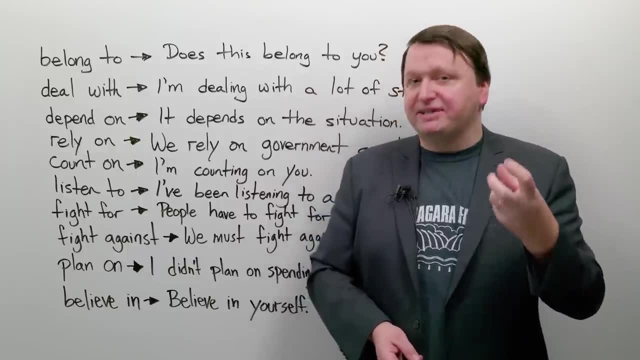 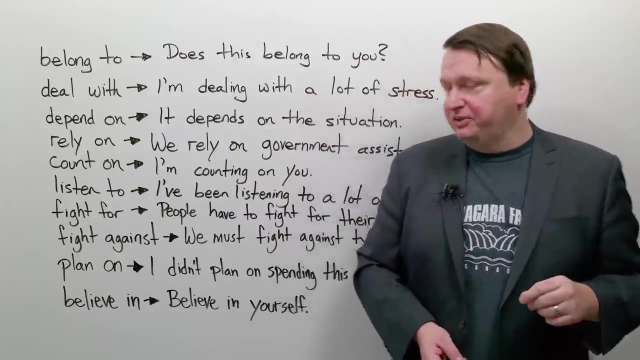 Rely on, Rely on, I'm counting on you. Good, So if you count on someone, you trust them to do something for you that they say they will do or they have promised that they will do for you. So if, for example, I can't think of a situation 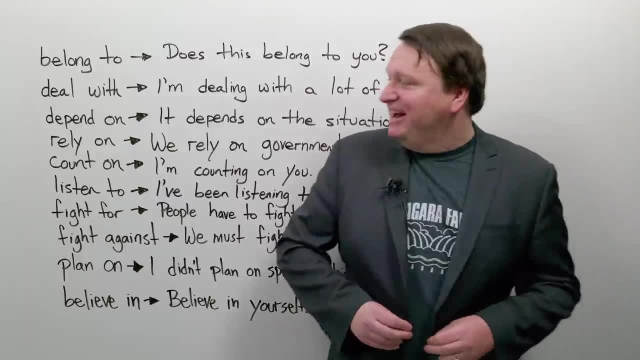 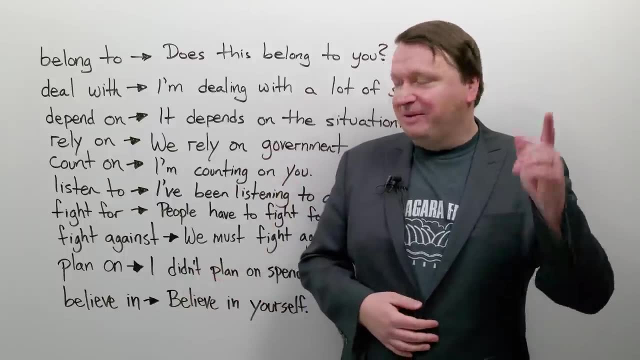 in the moment. It's so hard in the moment to think of one sometimes. So you can count on someone to do something for you. You trust them to do something for you. You trust them to do something for you, to do what they say they will do. i'm counting on you that you understand what i'm saying right now. 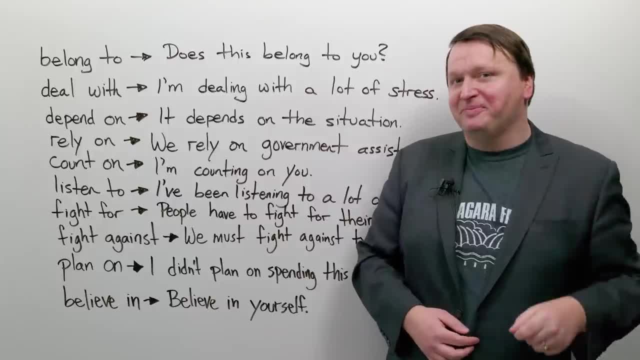 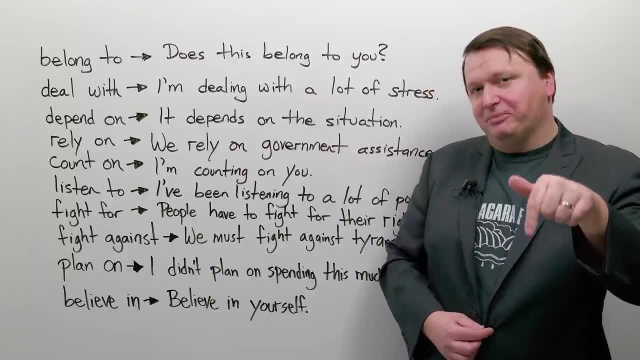 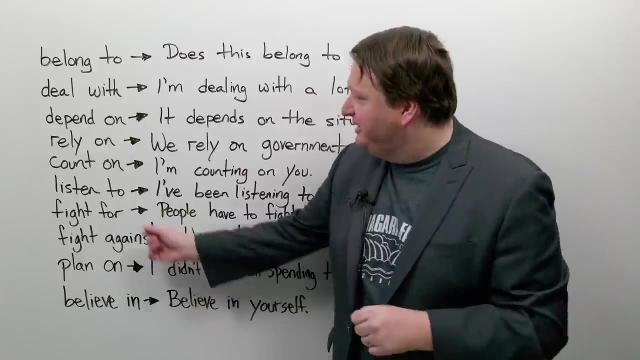 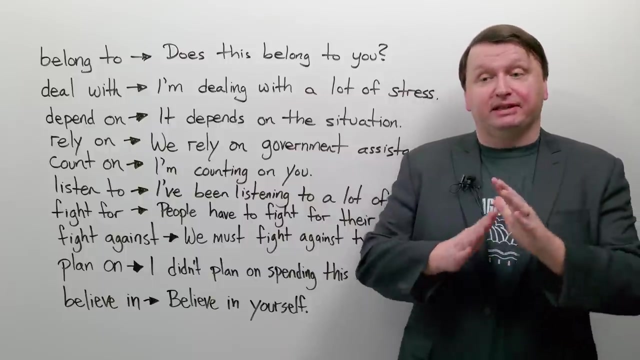 so one more time, repeat after me: i'm counting on you. okay, good, and you know what? give me a comment down below. what is a situation where someone might say this to someone: i'm counting on you. next, we have listen to. so a common mistake here is people say: just listen. for example, i listen. 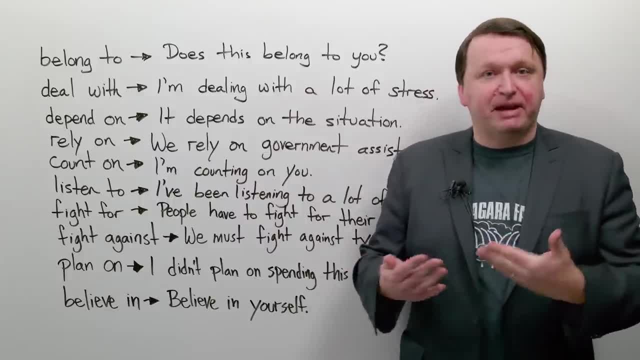 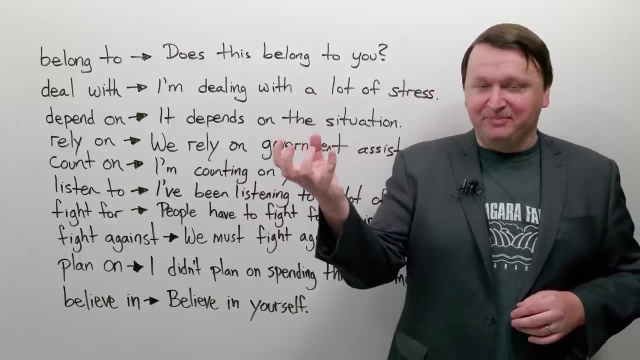 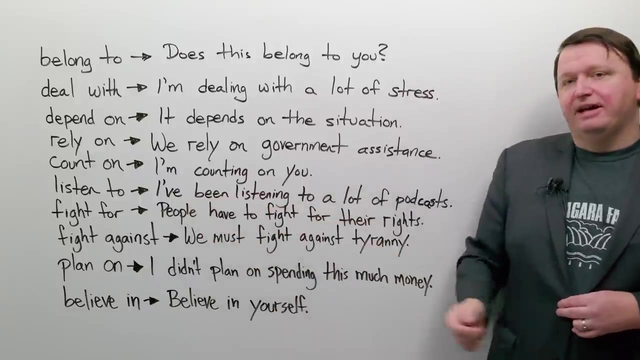 music, i listen podcasts, i listen my parents. uh, if you want to mention the person or the thing that is the object of your listening, you need to say you listen to that person or to that thing. so, for example, i've been listening to a lot of podcasts. 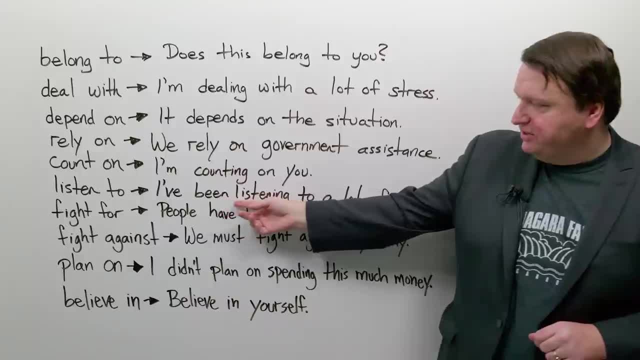 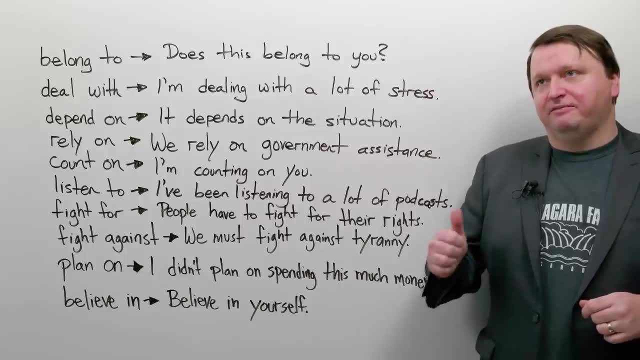 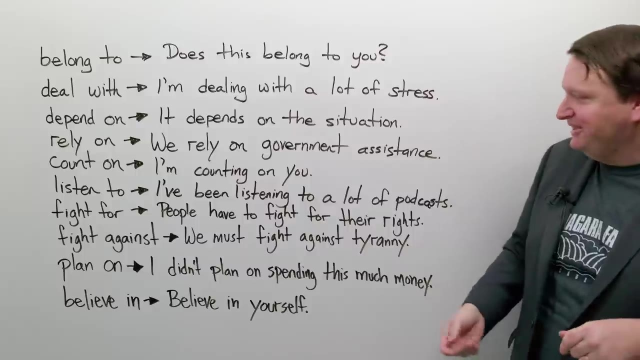 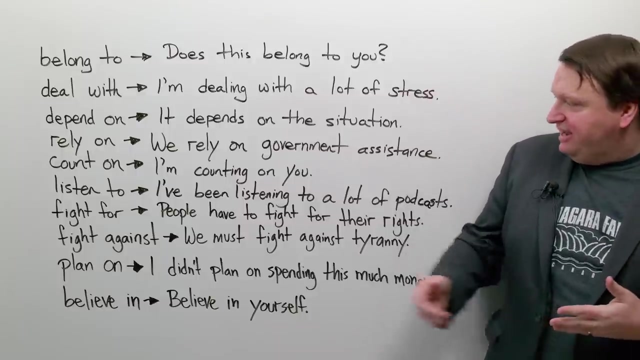 so again, you can listen to music. so repeat after me. i've been listening to a lot of podcasts. wonderful, you got the intonation and everything okay. next we have fight for. so if you fight for something, uh, here people have to fight for their rights. i just think of 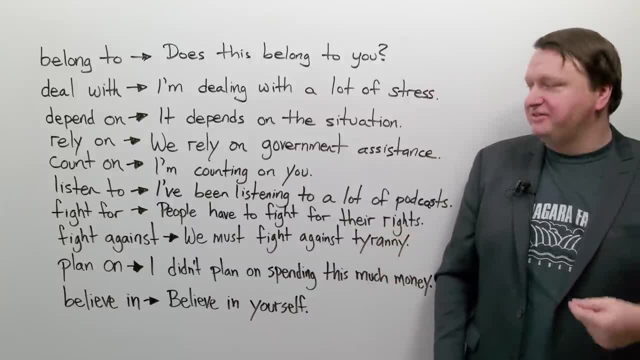 this as a common mistake. i've been listening to a lot of podcasts, so again, you can listen to music. so repeat after me. i've been listening to a lot of podcasts. old beastie boys song fight for your right to party, and if you are someone who was born in the 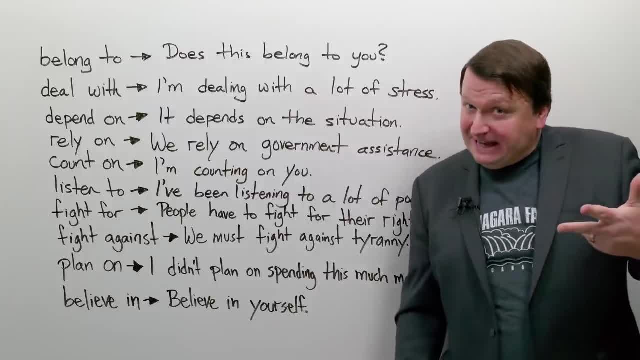 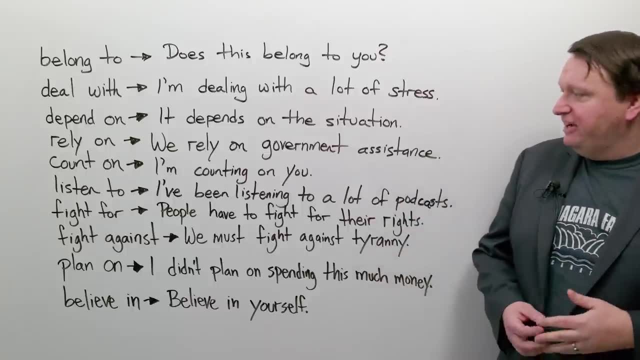 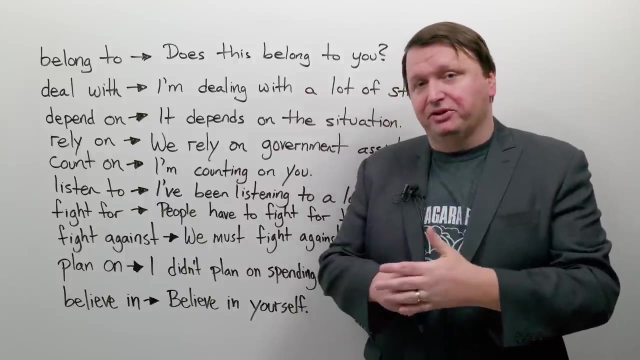 1970s, the 1980s, maybe the 1990s, you might know what i'm talking about. so you fight for something. fight for your beliefs, for your values, for your rights. you can also fight against something. so you're trying to push back against something. so we must fight against. 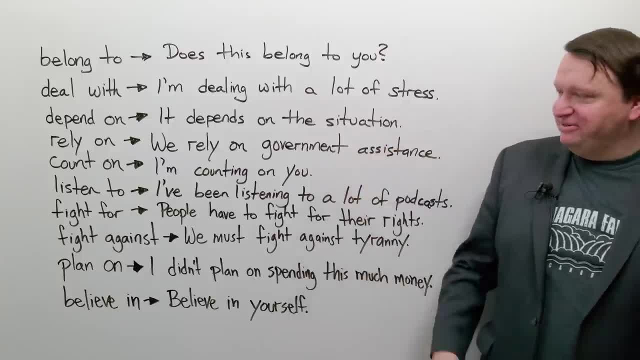 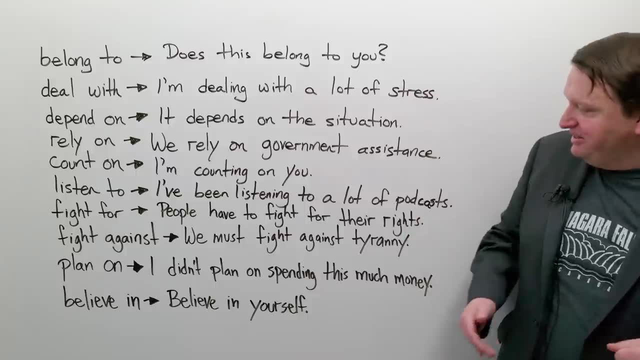 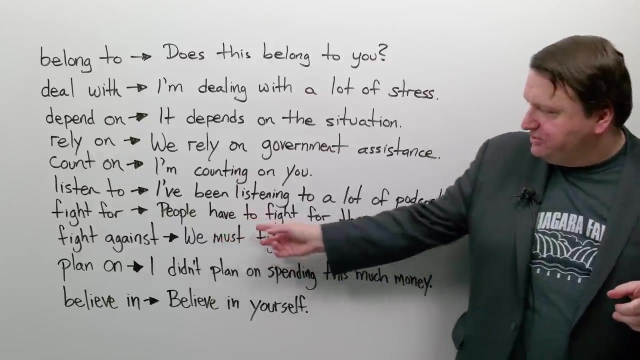 tyranny. uh, i have a lot of government examples here and tyranny and, you know, oppressive governments- um, not a great topic, but it's a reality in parts of the world. so we must fight against tyranny. uh, actually, repeat after me. first, we'll go with this one. people have to fight for their rights. 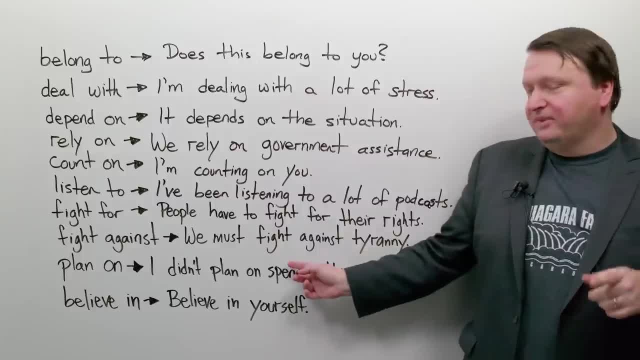 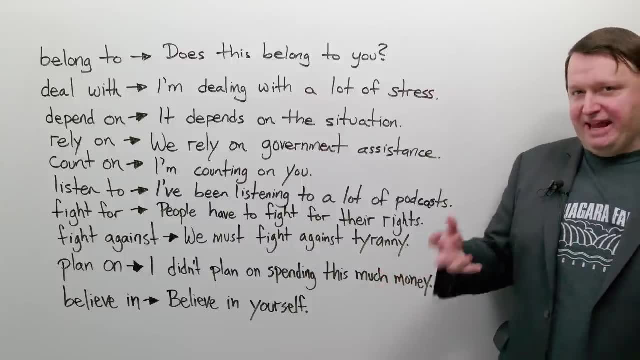 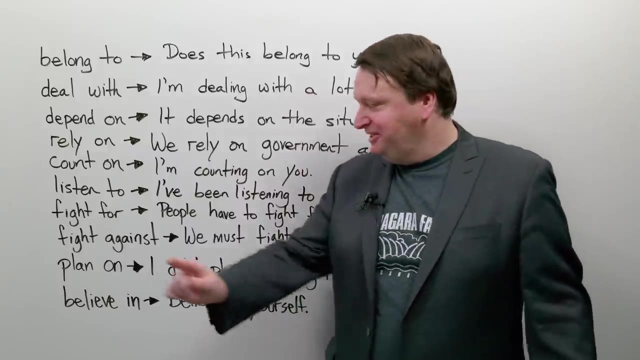 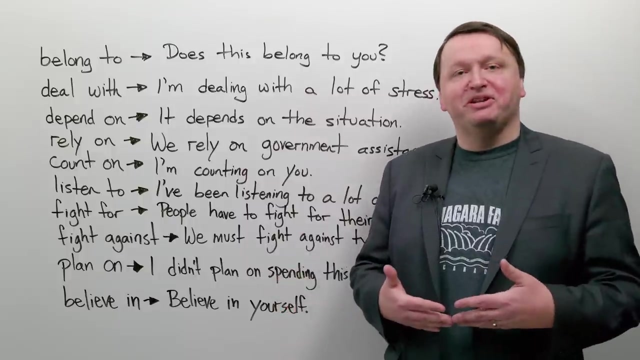 we must fight against tyranny now. i know this feels like an anti-government video now and i don't want it to feel that way, but these are the examples that came to my mind, i don't know why. next plan on: uh, so you can plan to do something, or you can plan on doing something. so, for example, i didn't plan on. 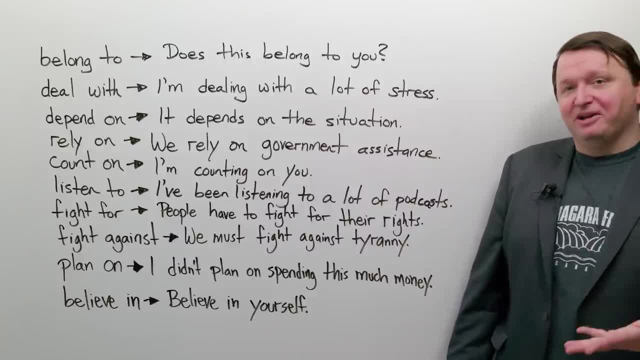 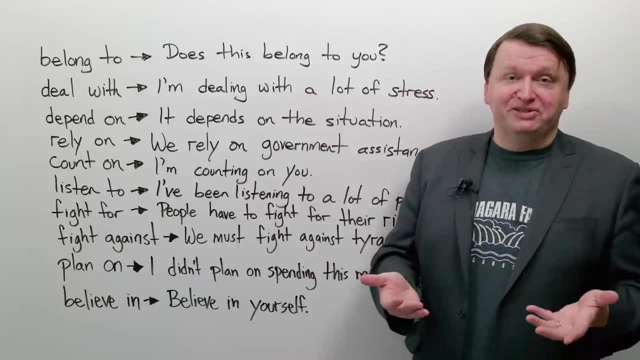 spending this much money. so you went to the mall. you saw that there were many sales and maybe you planned to do something. and you saw that there were many sales and maybe you planned to do something, planned on spending twenty dollars, but in the end you spent a hundred dollars and you said, oh my. 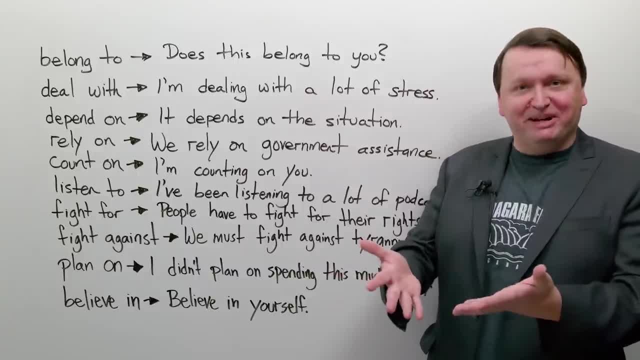 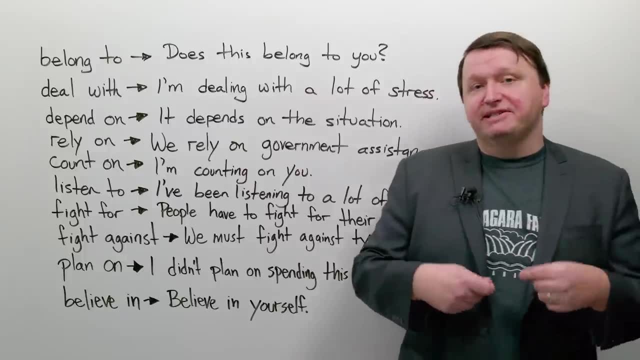 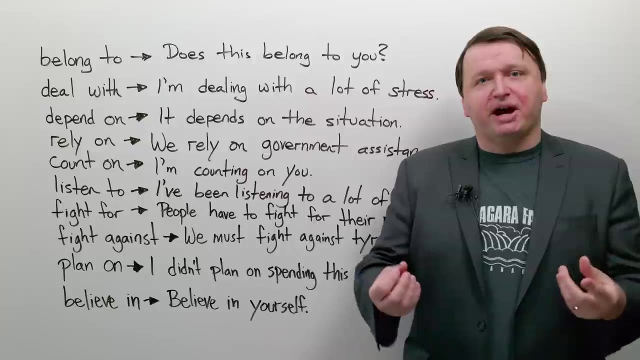 goodness, i didn't plan on spending so much money, so this wasn't my plan. next, believe in. so if you believe in something or believe in someone, you have faith in that person or faith in that thing. people talk about believing in god, believing in a cause. believing in a cause. 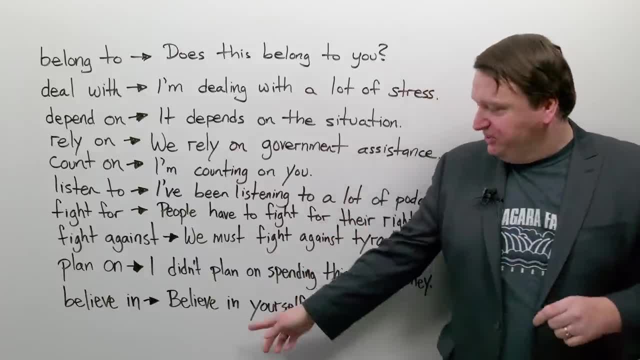 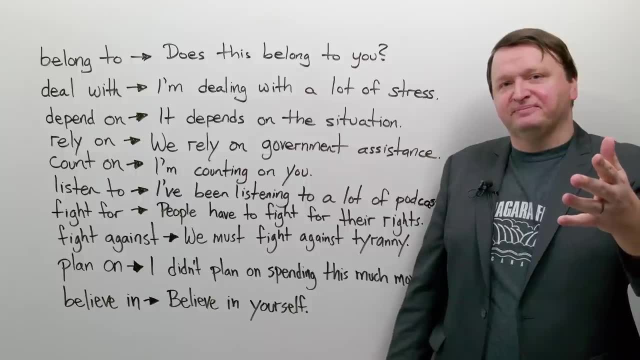 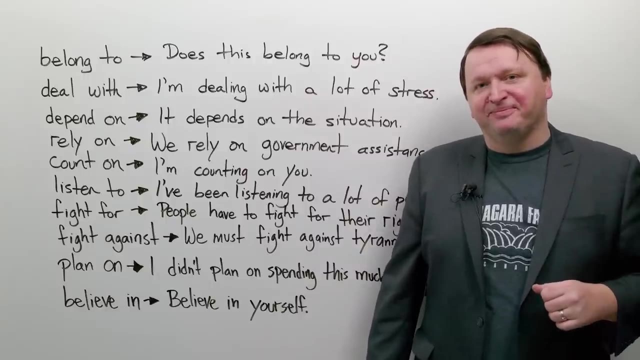 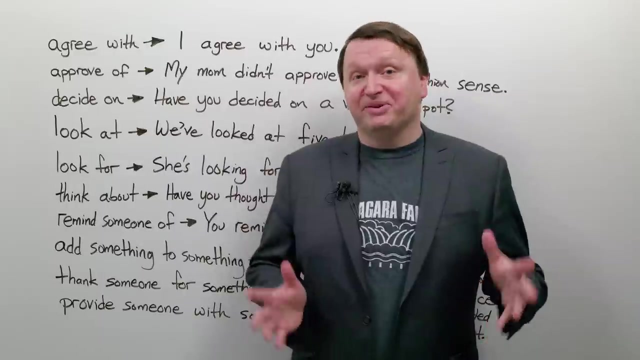 believing in yourself, believing in someone. so here we go. believe in yourself. so repeat after me: believe in yourself. and you know what? let's make this personal. repeat after me: i believe in myself. that's great, that's the spirit. all right, let's do 10 more, okay. so next up, we have agree with. 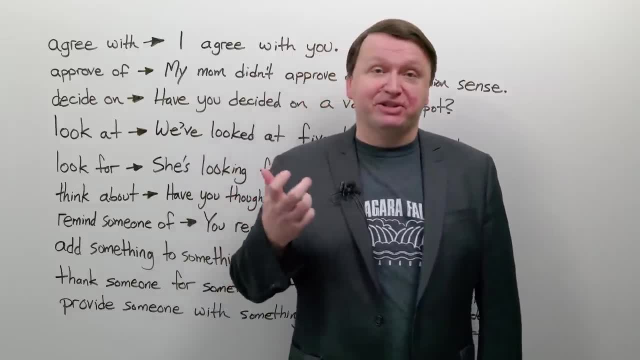 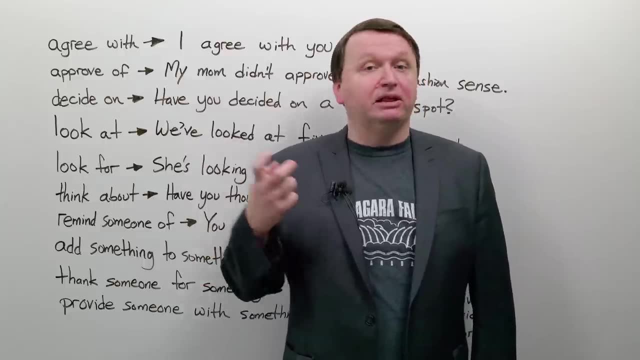 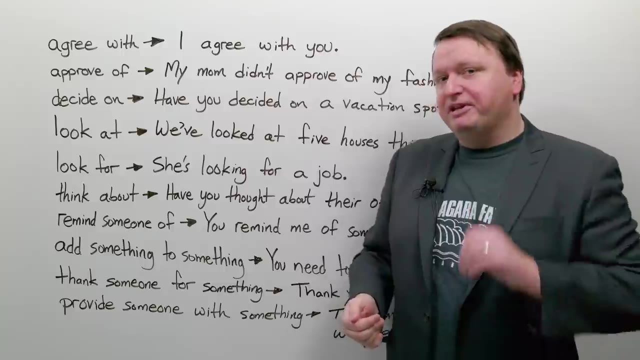 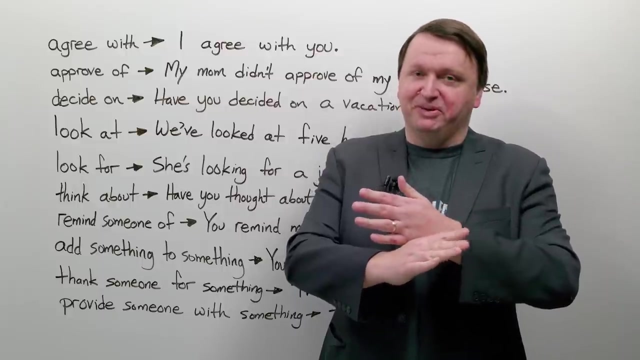 so you can agree with a person or believe in a person, or believe in a person or believe in a person with someone, or disagree with someone or something, for example. you can disagree with a policy or a law or a decision, for example, so i agree with you. a common error here is: some students say: i am agree, and i am agree is incorrect, so it's always subject verb, so repeat after me: i agree with you. 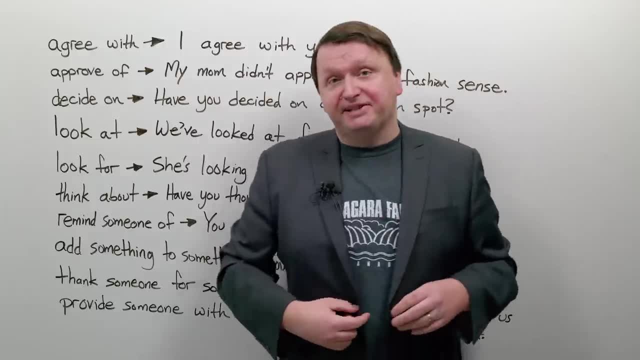 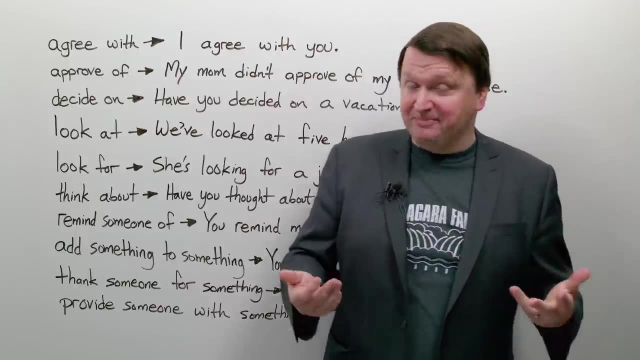 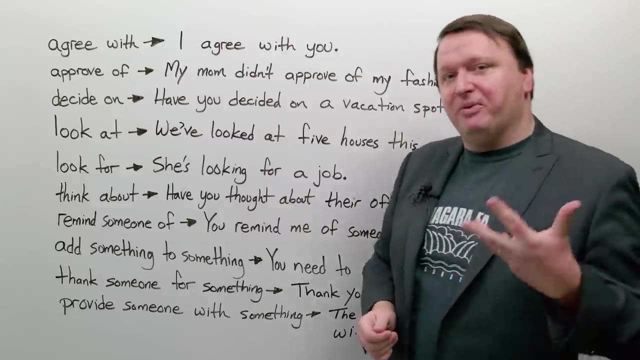 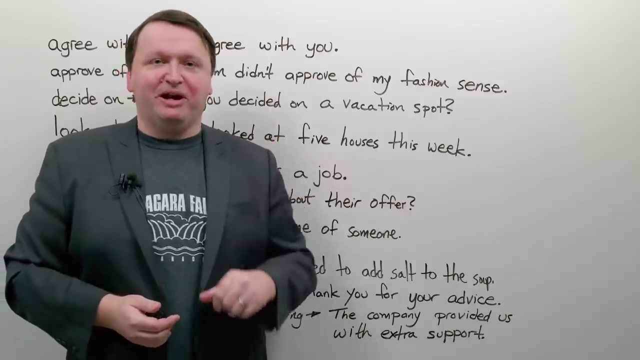 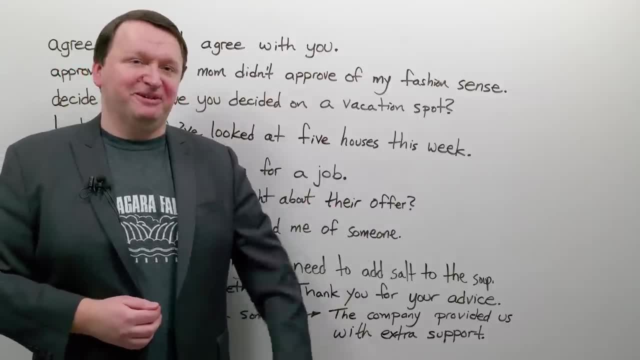 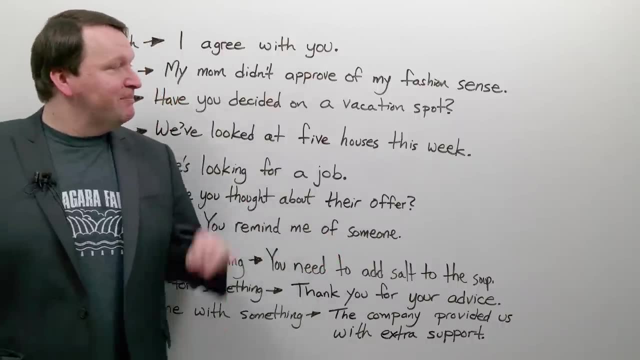 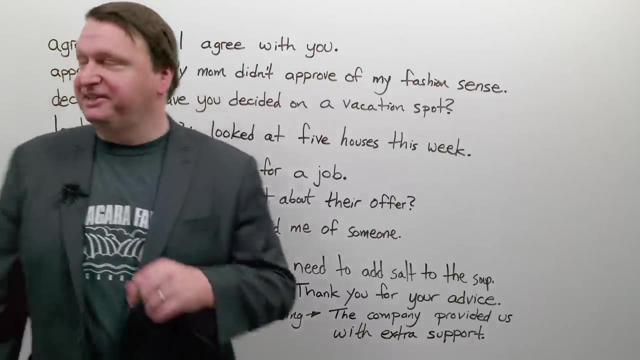 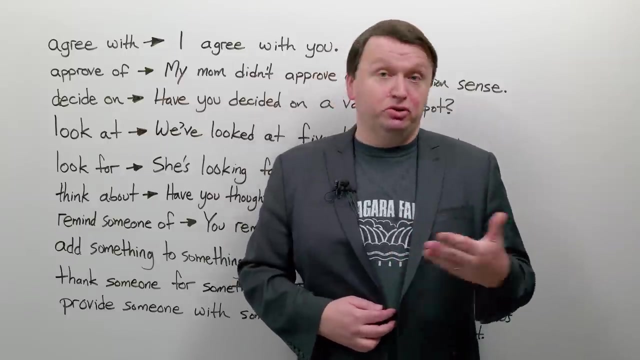 but I just want you to know I disapprove. So the opposite of approve is to disapprove of something. So repeat after me: My mom didn't approve of my fashion sense. All right, Good, Next we have decide on, So you can decide to do something. 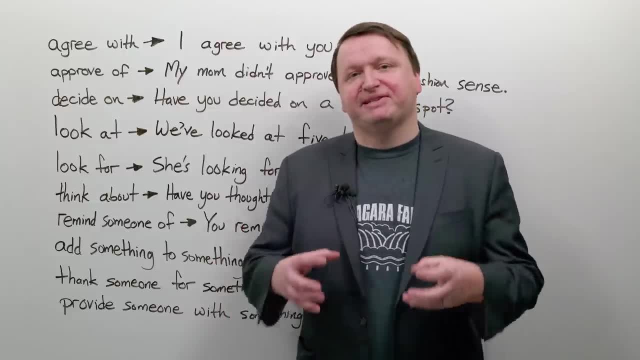 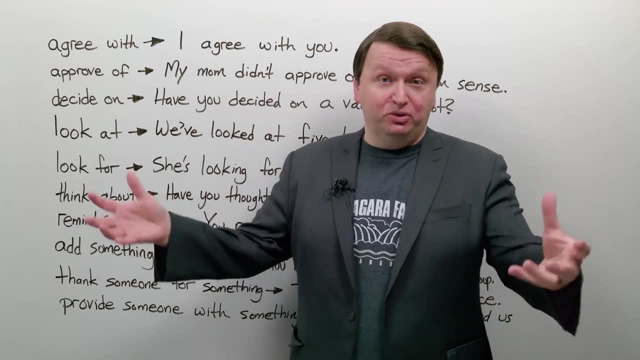 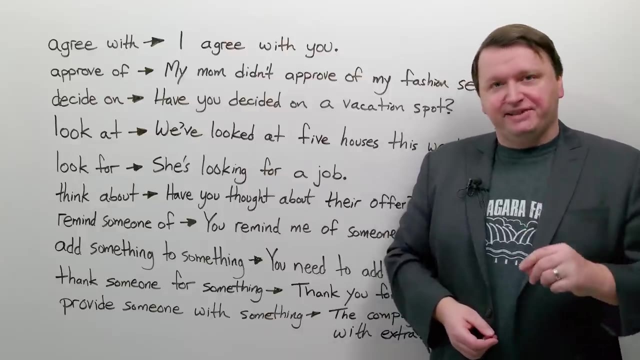 You can also decide on something. So you can decide on a plan, decide on a strategy, decide on what you're going to do. So, for example, have you decided on a vacation spot. So in this case, someone has told you that they are going on vacation with their family. 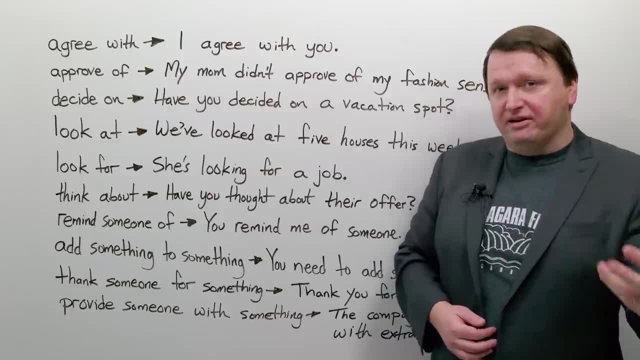 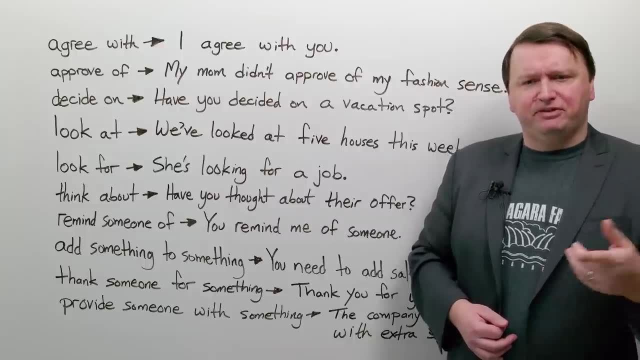 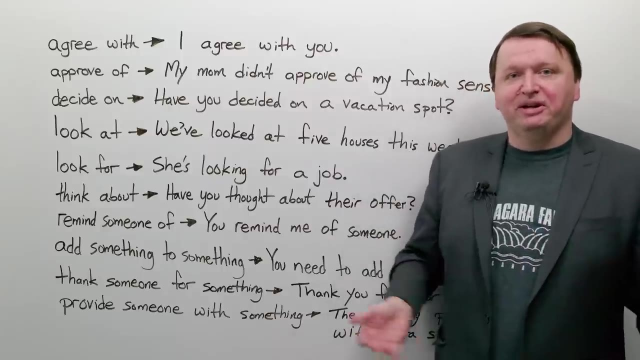 and they just haven't decided where they will go on vacation. And you talk to them three days later And you ask them: have you decided on a vacation spot? A vacation spot is the place of the vacation. So are you going to go, you know, to Mexico, to the Bahamas? 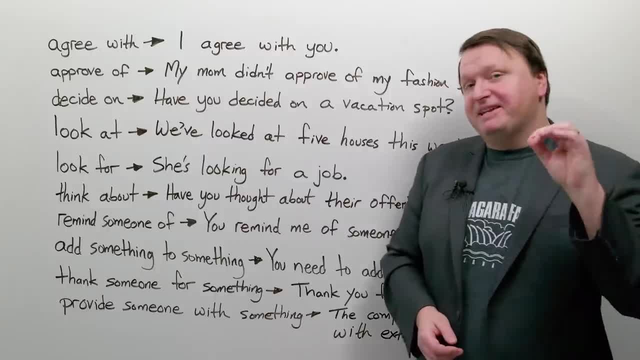 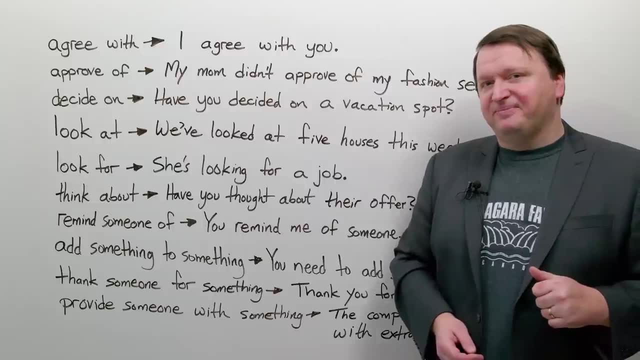 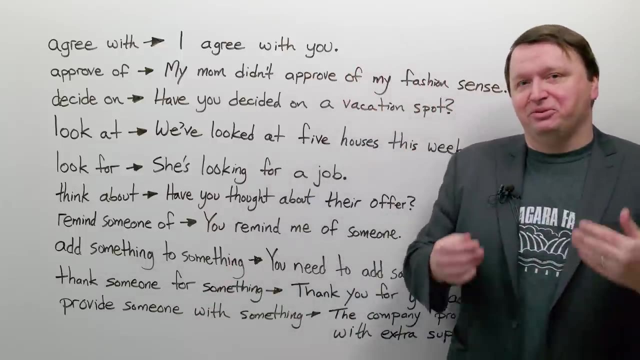 Or where are you going to go on your vacation? So repeat after me: Have you decided on a vacation spot? Next, we have look at, Look at. So you look At something, which means you direct your attention, the attention of your eyes, towards 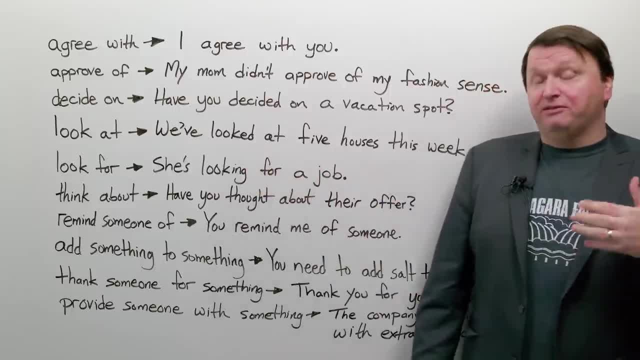 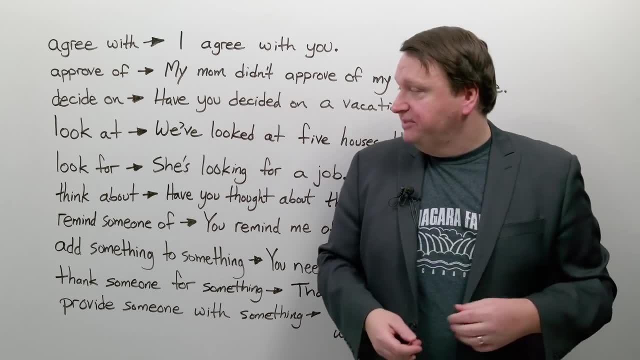 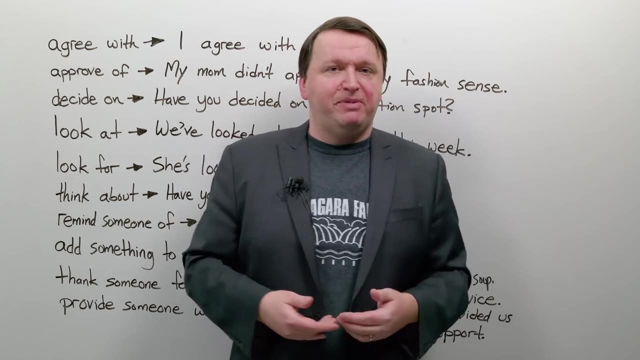 something or someone. So we've looked at five houses this week. So this person or this couple, these people are looking for a house and they have looked at five houses this week. Maybe they don't like any of them, or maybe some of them are too expensive. 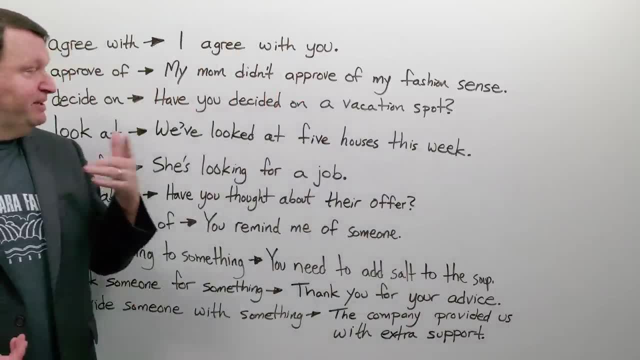 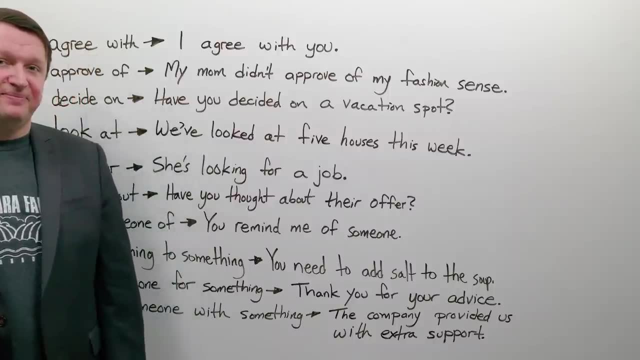 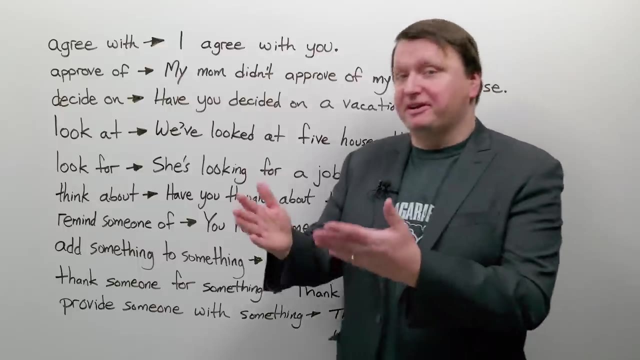 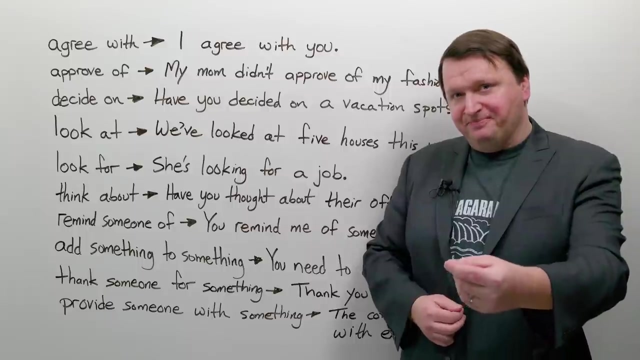 So imagine you are house shopping And repeat after me: We've looked at five houses this week. Okay, very good. Next you can look for something to search for something. So here she's looking for a job. So she is checking the online ads. 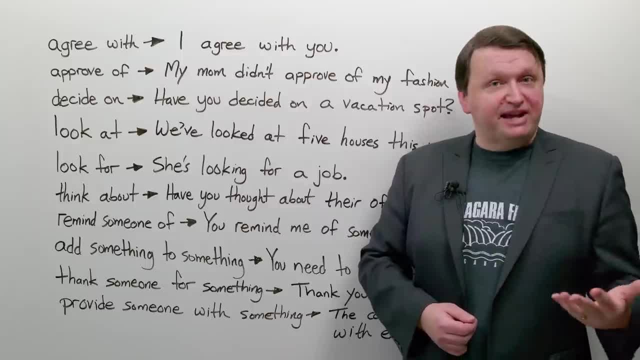 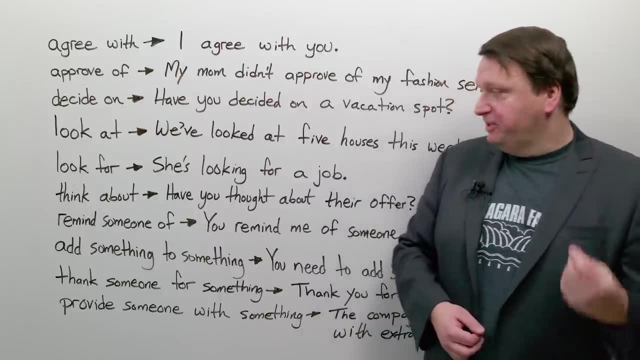 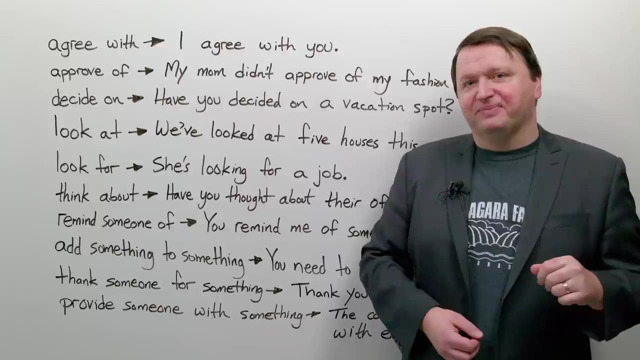 Maybe she is checking the newspaper. Maybe she is asking her friends If they know anyone at their company who might be willing to give them a job, for example. So repeat after me: She's looking for a job. Good, So we look for things online all the time. 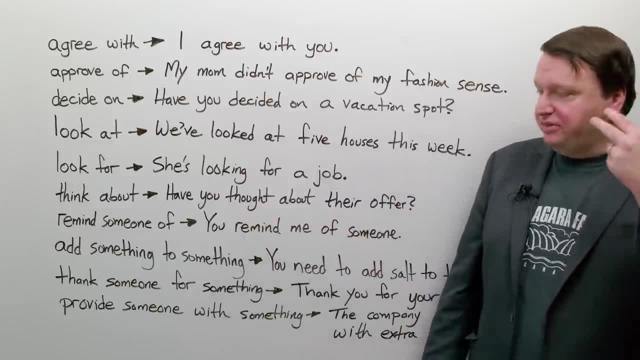 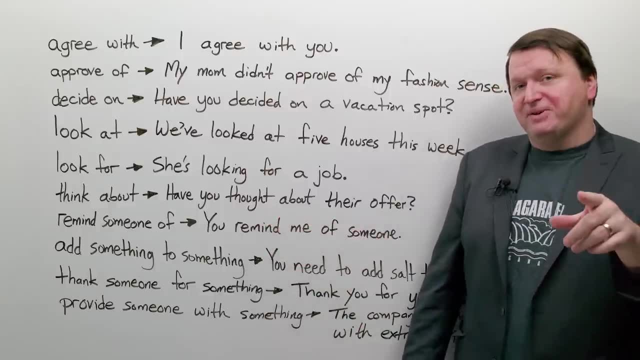 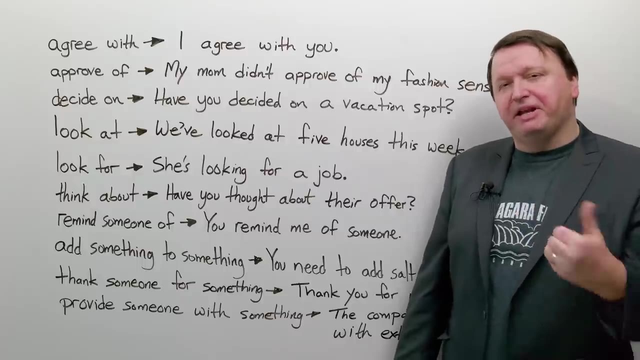 Next think about. So you're giving your thought to something and you're considering something Have you thought about? Have you thought about their offer? So this person is asking if you have thought about a job offer, maybe from a company, or your company wants to give you a promotion. 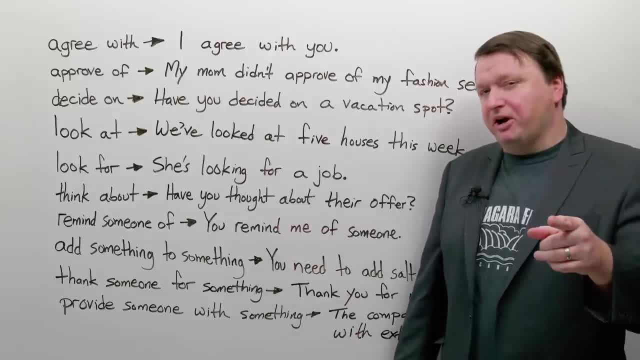 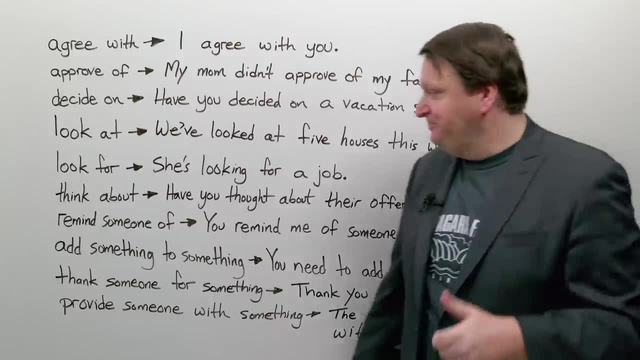 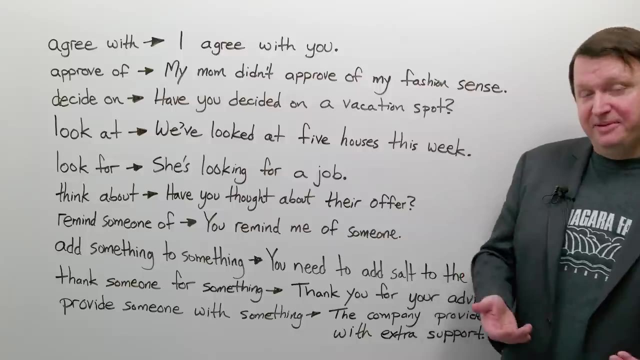 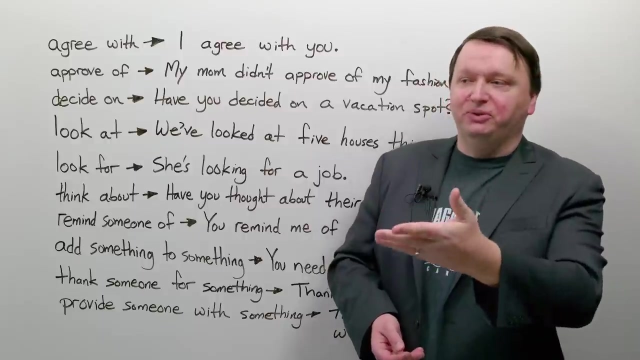 So repeat after me: Have you thought about their offer? Good, And next we have remind someone of something or someone. So if you remind someone of something or someone, you think. when I look at you, I think of this person or that thing. 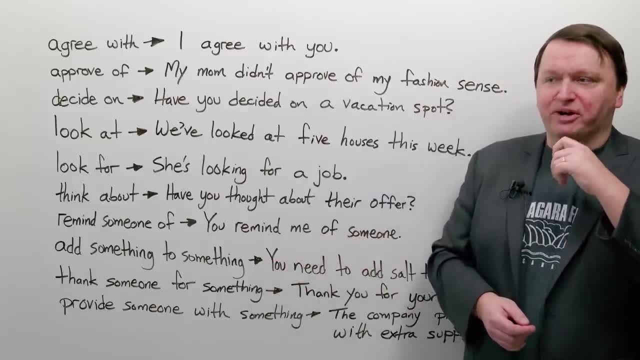 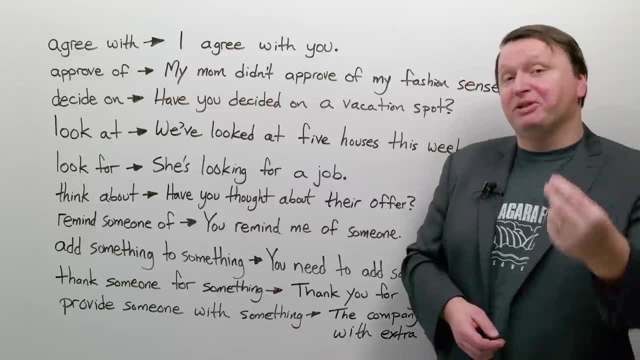 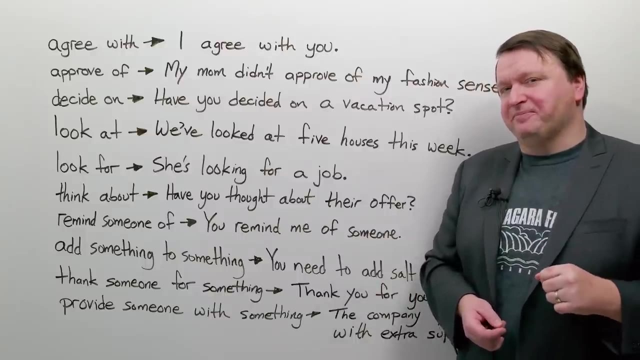 So, for example, you remind me of someone. Like you have a similar character to another person, or maybe you look similar to another person that I know, So repeat after me: You remind me of someone. Good, Okay, So you remind me of someone. 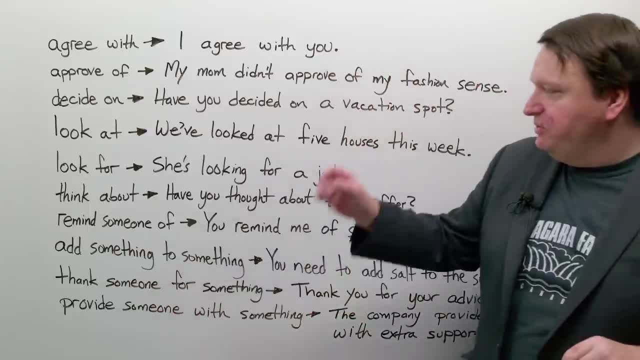 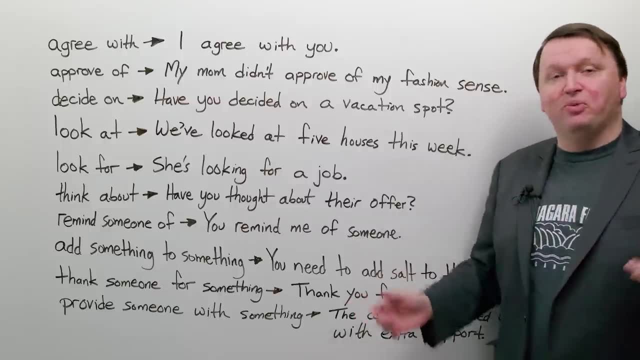 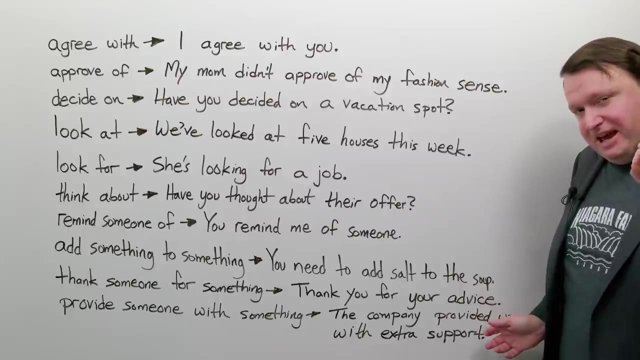 Well done, And we only have three more to go. So you can add something to something. So you can. when you're cooking, you add ingredients to what you are cooking, So here you need to add salt to the soup. So repeat after me. 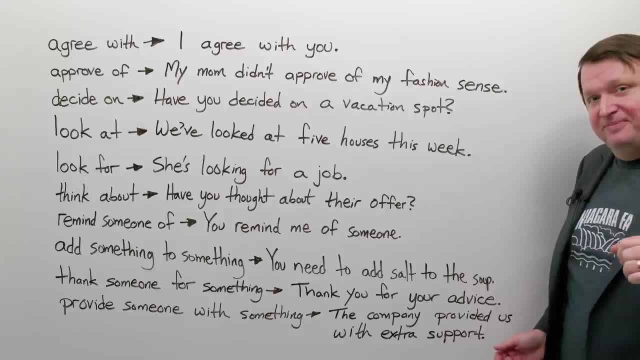 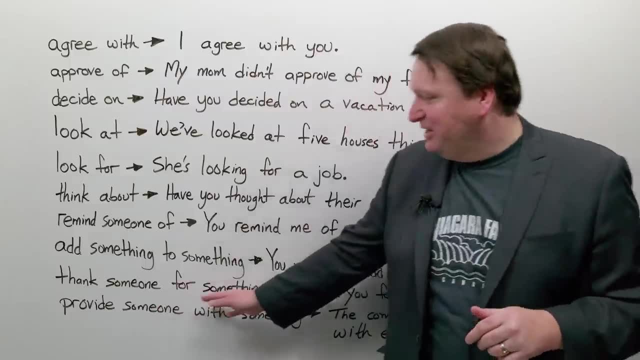 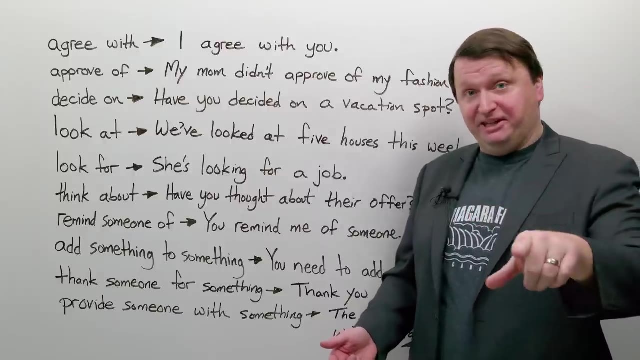 You need to add salt to the soup. You got it Good, So you remind someone of something Good, Okay good, And you can also thank someone for something. So I want to thank you for watching this video And, if you like it, don't forget like, share, subscribe EngVidcom. do the quiz? 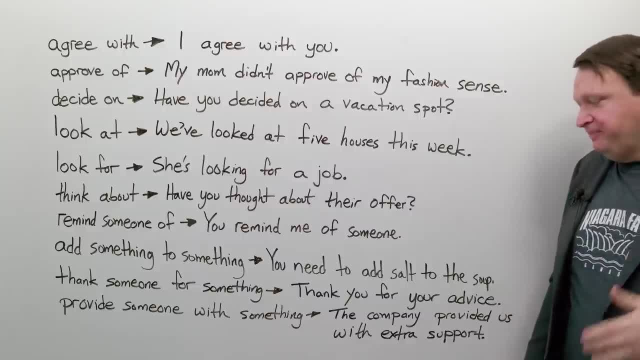 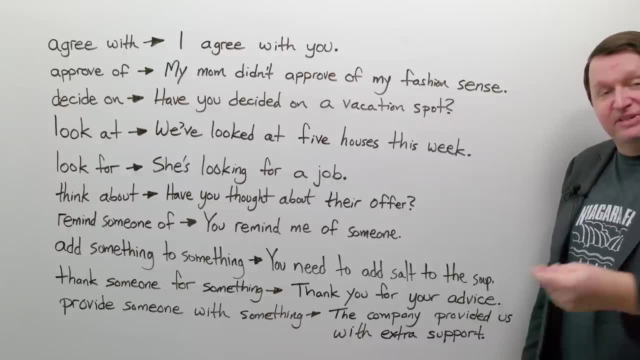 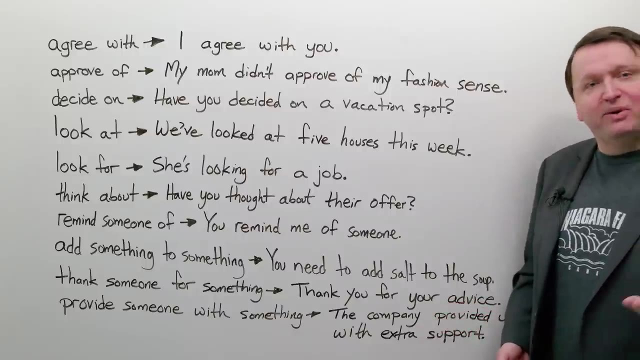 So here another sentence. Repeat after me: Thank you for your advice, Thanks. So in this sentence you are showing gratitude to someone for something. In this case you are showing gratitude for the person's advice. And finally, you can provide someone.